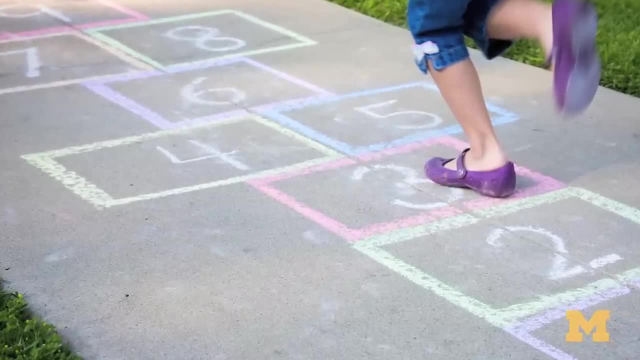 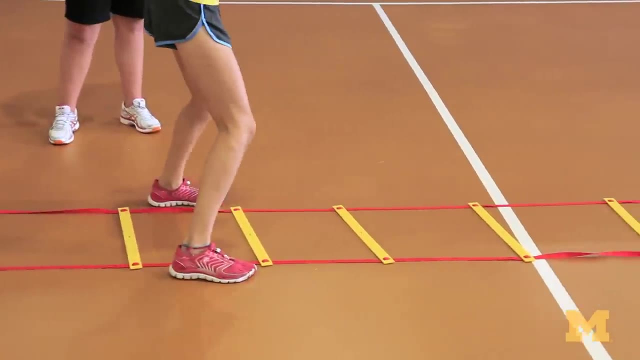 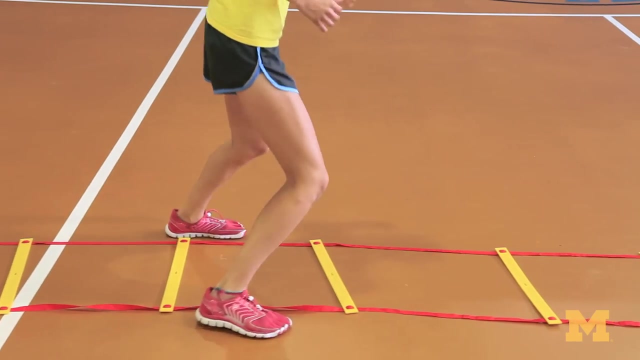 with sidewalk chalk, or you can use an agility ladder, like we're going to use today. Start by jumping with two feet out and hopping to one foot, And you can use the same foot throughout as you're starting to practice. So, for instance, you're going to go with two feet, then hop on left foot, two feet, hop on right foot. 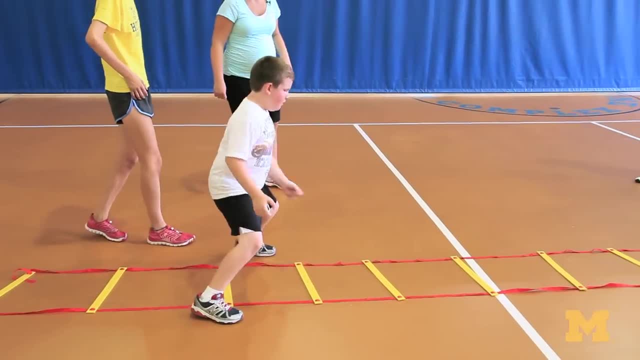 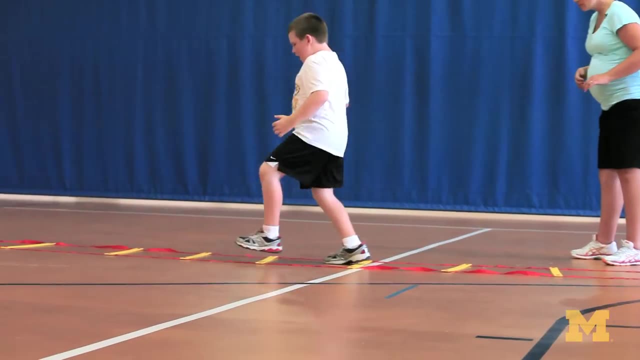 If that's too difficult for your child, you can just start with two feet jump on left foot. two feet jump on left foot until they get the feeling of the correct movement while going through the hopscotch grid. Some other activities that you can do through the agility ladder would. 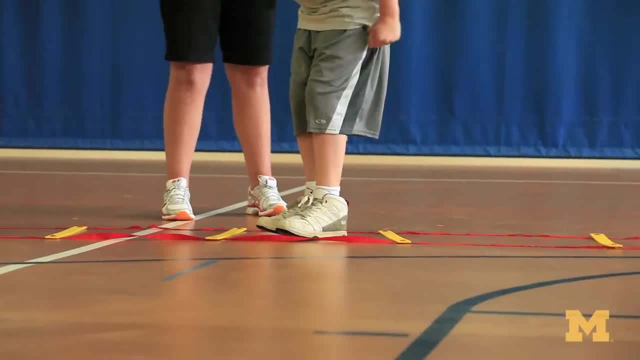 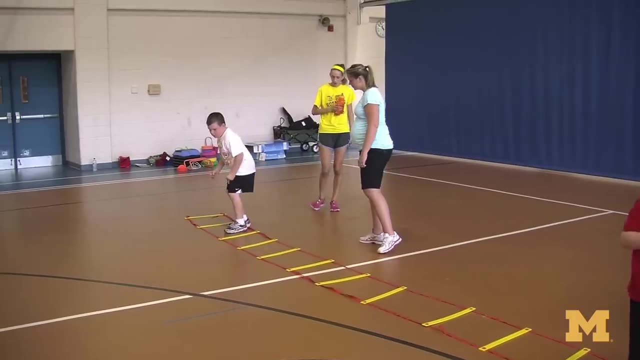 be jumping with two feet forward, two feet backward, two feet forward, two feet backward or two feet side to side. Those are great activities working on keeping both feet together, and you can use the cues for gluing your feet together so that they don't come apart while 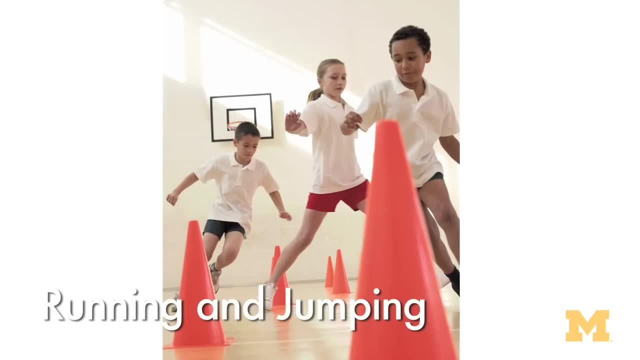 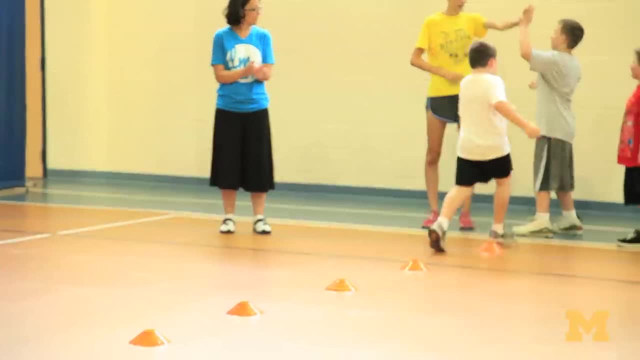 jumping over the lines. Another great activity would be running in and out of cones. You don't have to have cones. You can use paper cups or plastic cups or even paper markers that you can place on the floor. You can run in and out using a figure eight pattern. You can run backwards. 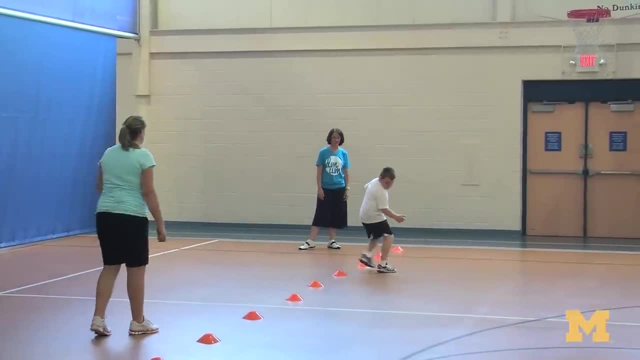 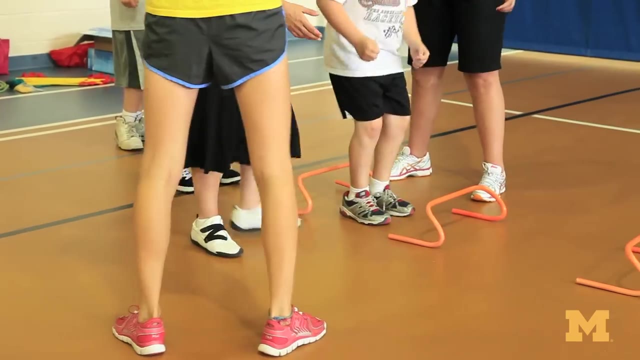 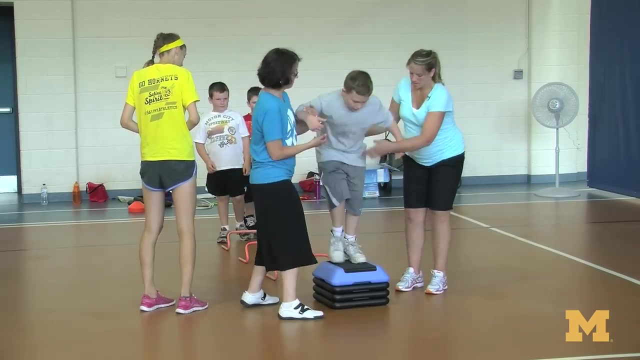 through the cones using the figure eight pattern to increase the difficulty. Jumping with two feet over hurdles can be a really challenging task for kids, but it's great for coordination and strength. You can use books or you can use any other object. that's about six inches off of the floor and jump with two feet over the top of each of the hurdles. 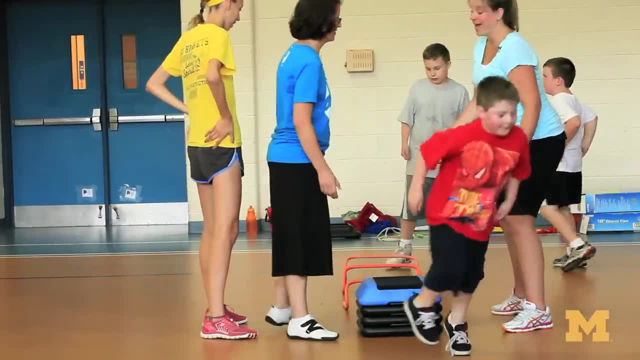 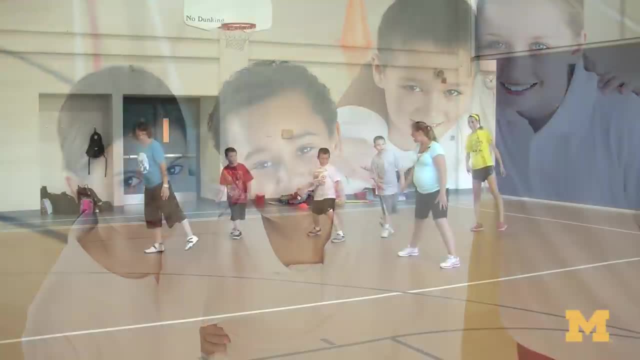 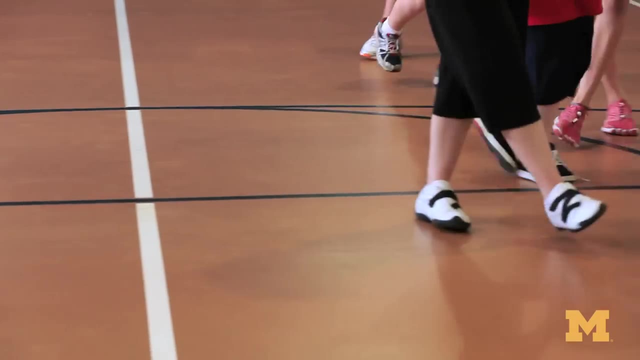 At the end jump onto a solid surface and jump off of the solid surface to work on landing and form. So the last activity we're going to participate in is karaoke. Start by facing your body and then stepping forward, with your left foot stepping over the top, with your right foot stepping with 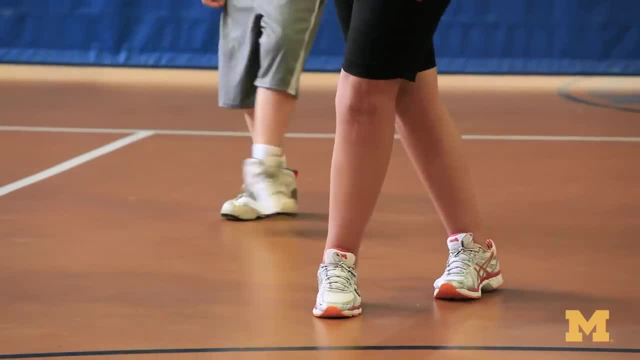 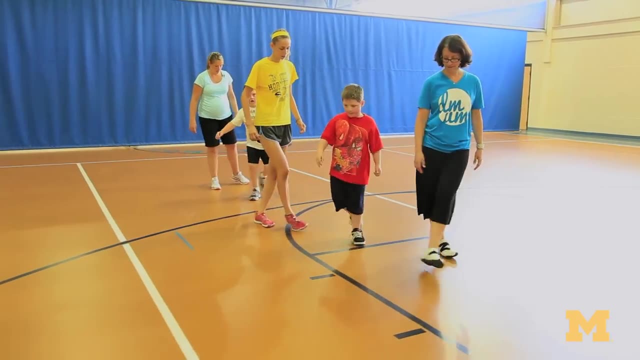 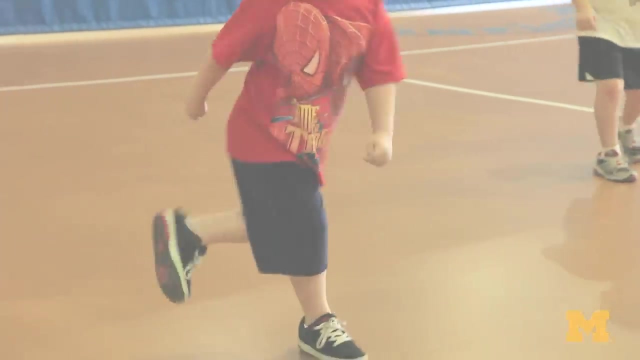 your left foot again and right foot behind. So you're going to go left foot right over, left foot right behind. Move in both directions so that your children can work on bilateral movements and strengthening in both directions. Thank you for taking the time to learn new tips. 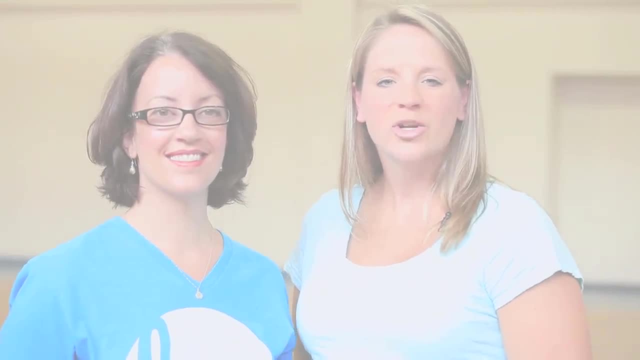 to help your children with agility and endurance. For more tips, visit the website at wwwmottchildrenorg. slash camp.